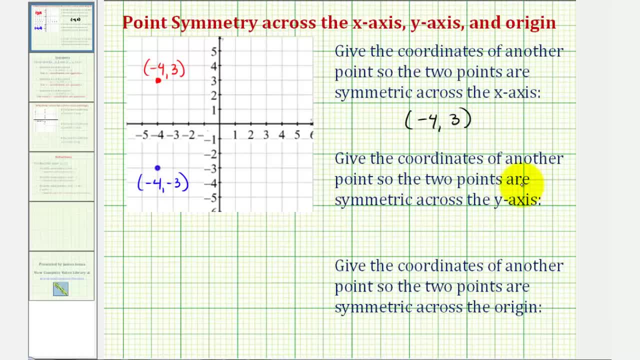 Now we want to give the coordinates of another point. so the two points are symmetric across the y-axis. We'll notice how the given blue point is four units to the left of the y-axis. So if we reflect this point across the y-axis, so the two points would be symmetric across the y-axis. 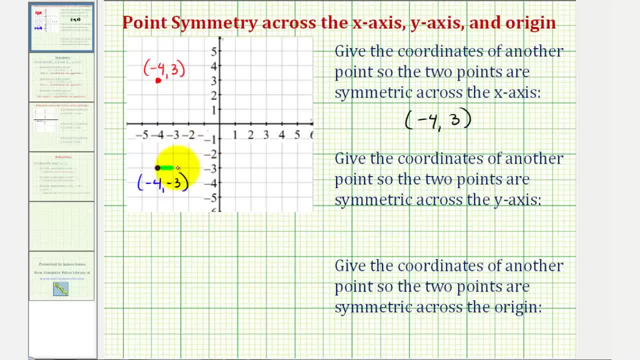 the new point would be four units to the right of the y-axis here. Notice how the coordinates of this point would be positive four comma, negative three. So when two points are symmetric across the y-axis, notice how the y-coordinates would be the same. 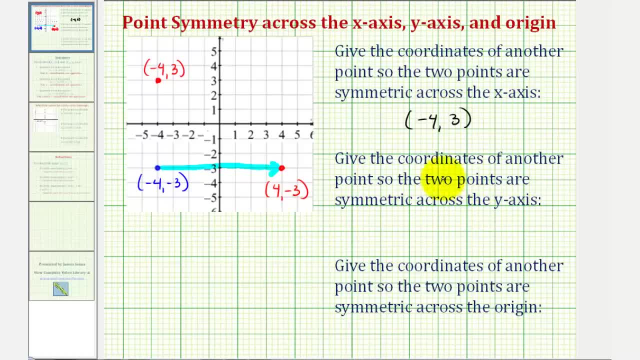 but the x-coordinates would be opposites. So the coordinates here would be four comma negative three. And now, finally, we want to give the coordinates of another point. so the two points are symmetric across the origin. So to find the coordinates of the second point, 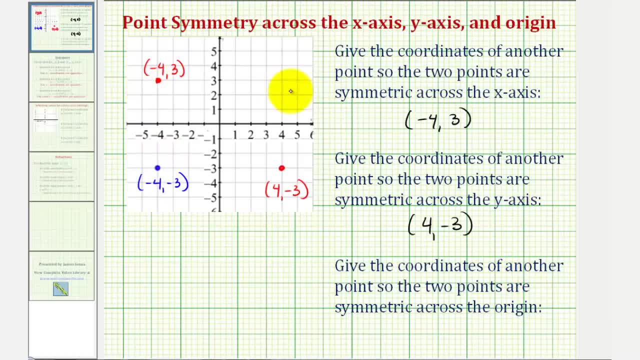 we want to reflect the given point across the x-axis and the y-axis. So if we take the given blue point and we reflect it across the x-axis, we already know it would be here. But now, if we reflect this across the y-axis, 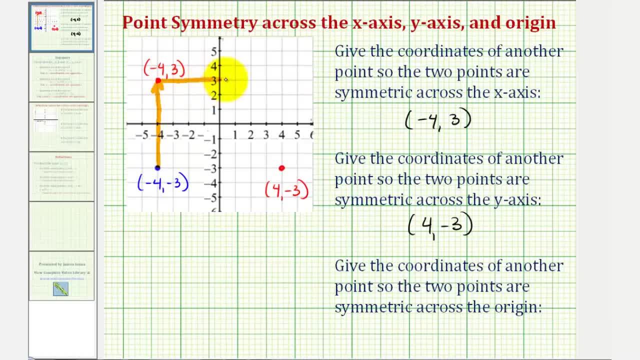 the new point will be four units to the right of the y-axis, which would be here. So the coordinates of this point notice would be positive four comma, positive three. So if two points are symmetric across the origin, notice how the x-coordinates and the y-coordinates 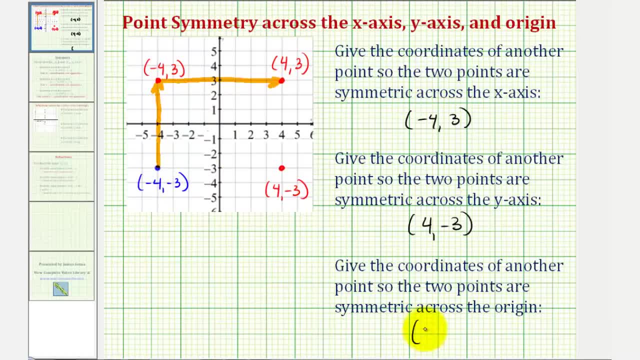 are opposites. So this last point would be four comma three. Another way to think of two points that are symmetric across the origin would be to take the given point and rotate it about the origin 180 degrees. So if we took this blue point here, 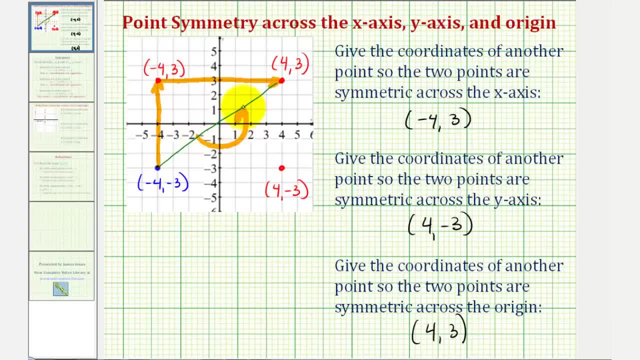 and rotated it 180 degrees about the origin. notice how it would give us this red point which is symmetric across the origin. So, to summarize what we did here, I'll leave you with this. I'll leave you with these notes here. I hope you found this helpful.